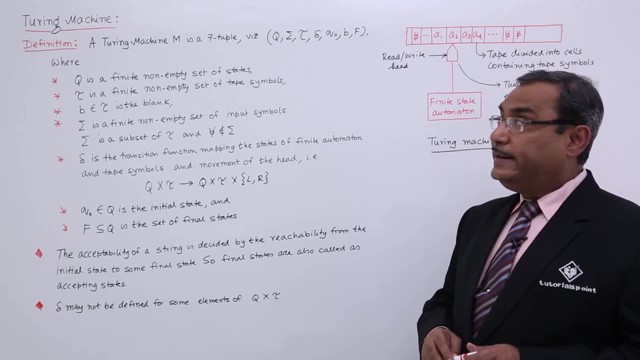 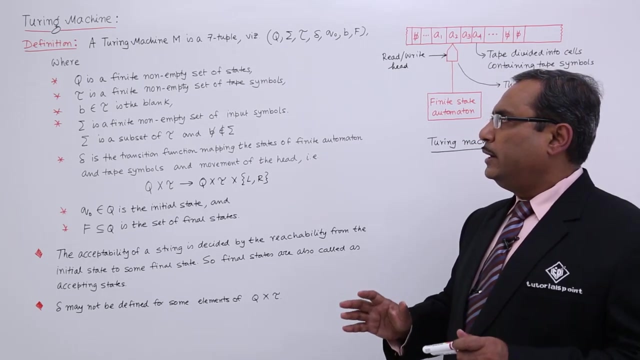 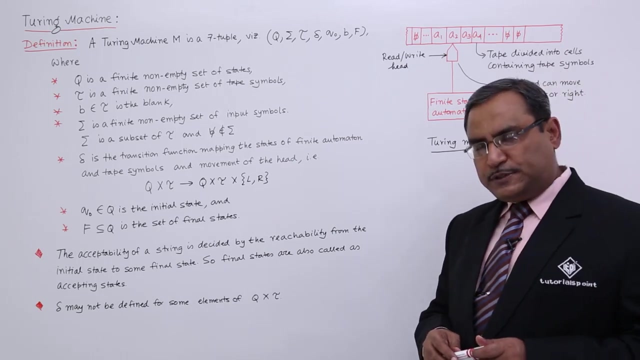 these are the 7-tuples. are there Now let me explain each one of them. What is Q? That is quite well known. Q is a finite, non-empty set of steps. What is tau? Tau is a finite, non-empty set of tape symbols. So there will be one tape and the tape will have different 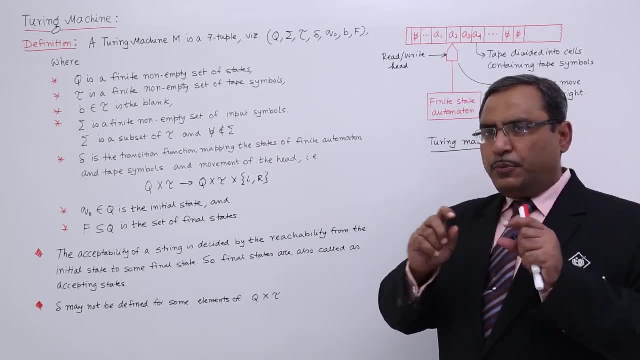 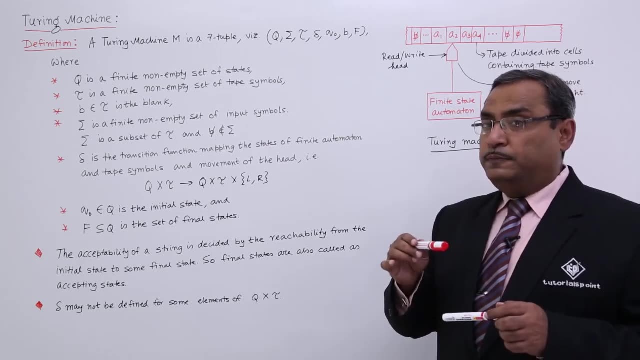 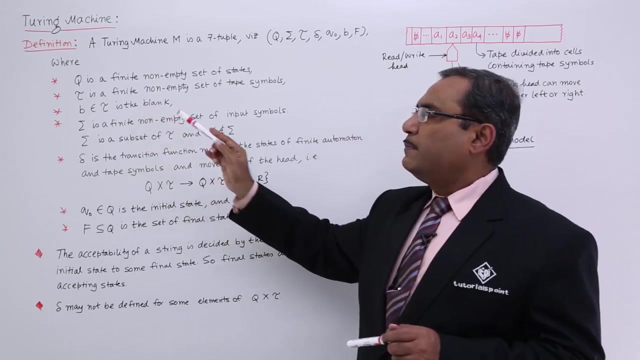 cells and at different cells will be having some symbols and all those symbols set will be kept in tau and out of those symbols one symbol will be blank. So B is an element of tau is a blank, So B is a blank. So this blank is this B and sigma is a finite, non-empty. 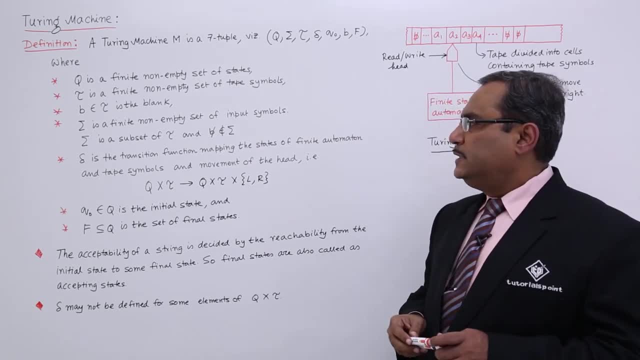 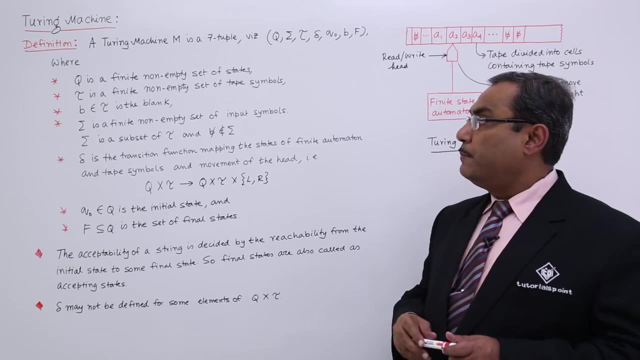 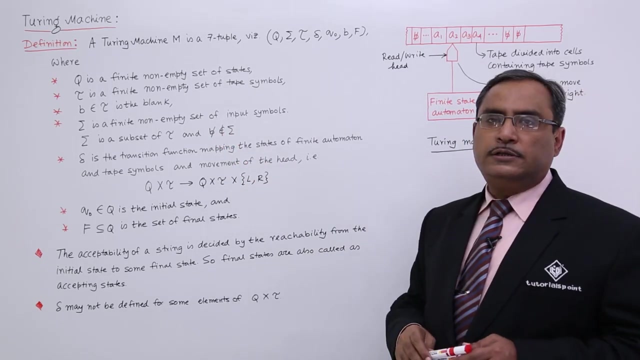 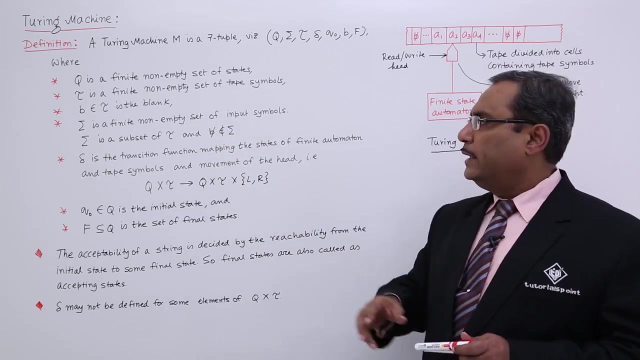 set of input symbols or input alphabets. Sigma is a subset of tau. That means sigma will contain some of the tape symbols, but sigma cannot contain blank character. So blank is not a subset of, is not is not a belonging to sigma. That means blank is not included in sigma. So that is our definition of Q. 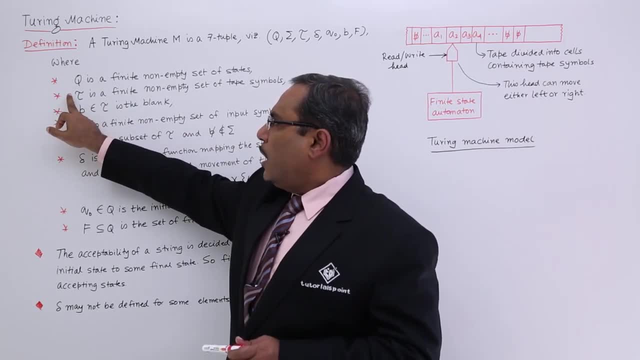 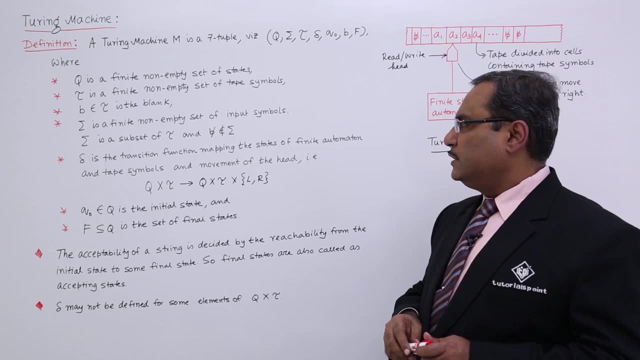 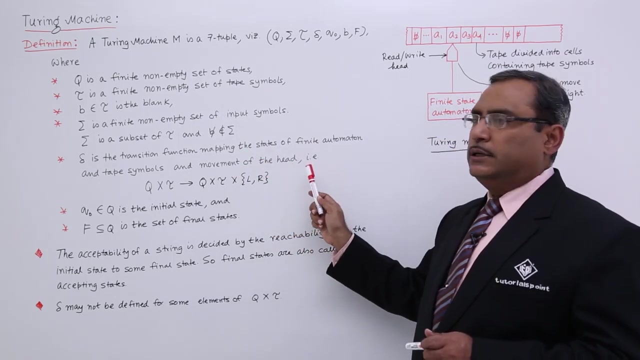 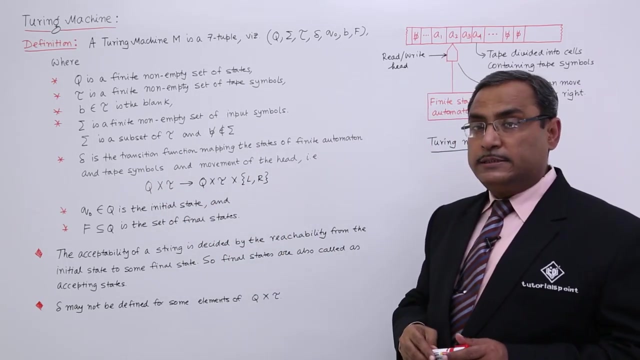 tau, B and sigma. Now we are going to discuss delta. Delta is the transition function mapping the states of the finite automaton and tape symbols and movement of the red-red head. So, as example, Q cross, tau, that means what is cross? Cross means Cartesian product. What is Q? That is? 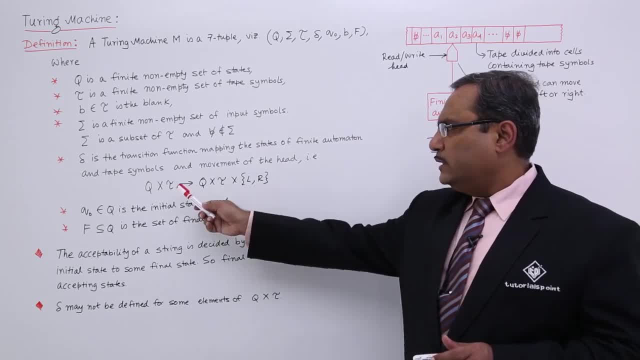 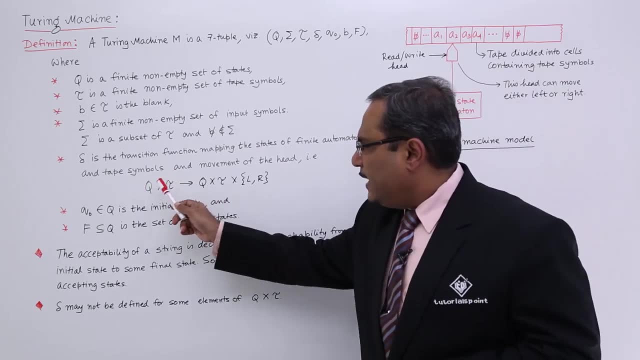 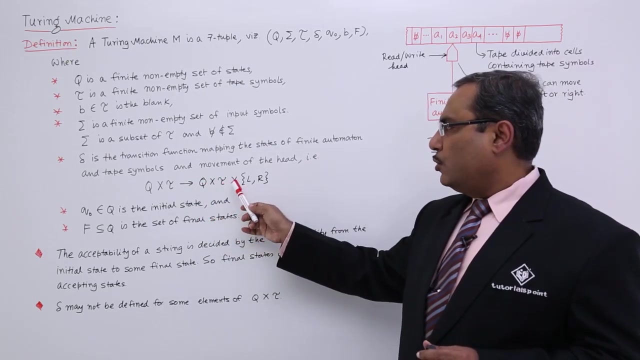 q, that is a set of states. what is tau? that is a set of tape symbols. So what is q cross tau? that means state and tape symbol, all possible combinations which will map on to q cross tau, cross l r. what is l r? l stands for left and r stands for right. that means after reading. 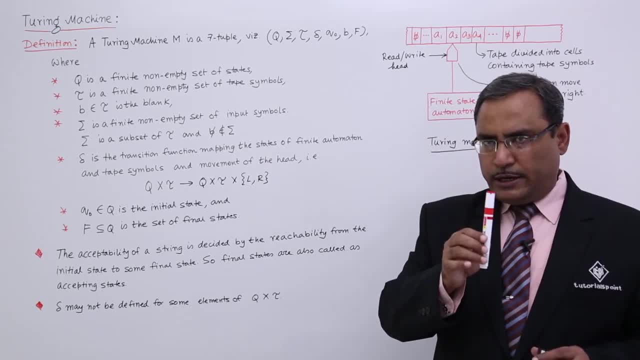 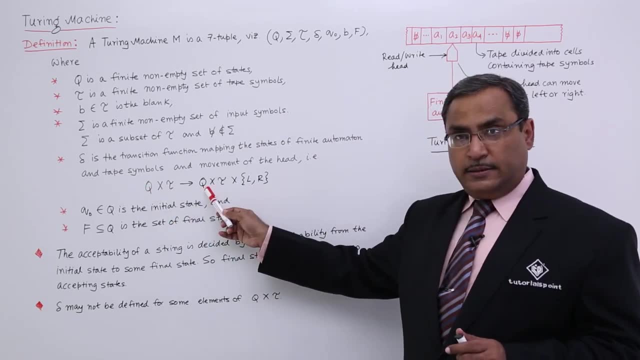 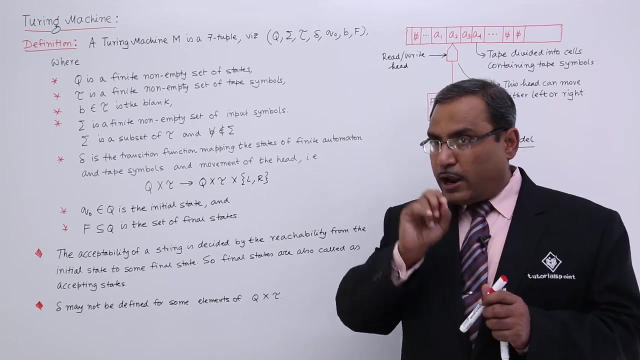 the input string and, depending upon the tape symbol and the current state, it will go to the next state. may be the. these two states might be same, So it will go to the next state. at what symbol it is going to write to that particular cell. So that is a tau. 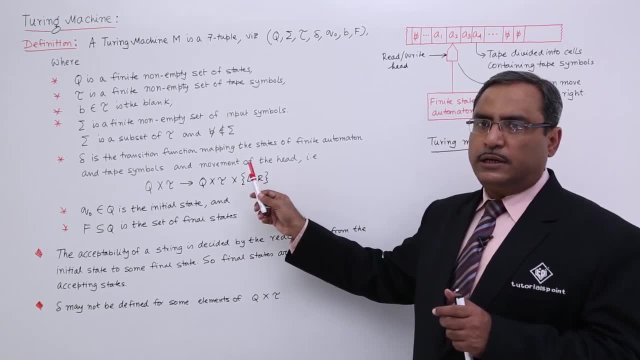 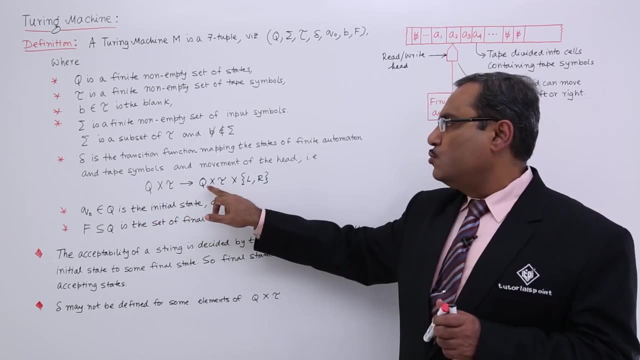 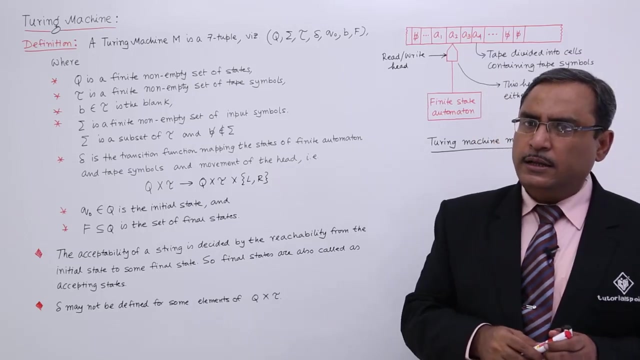 that is a tape symbol, and whether it will move towards the left or towards the right, that will be there. So q cross tau Tau maps into q cross tau, cross l r. So in this way, delta has been defined. what is delta? Delta means the transition function. q. 0 belongs to capital, q is the initial state. 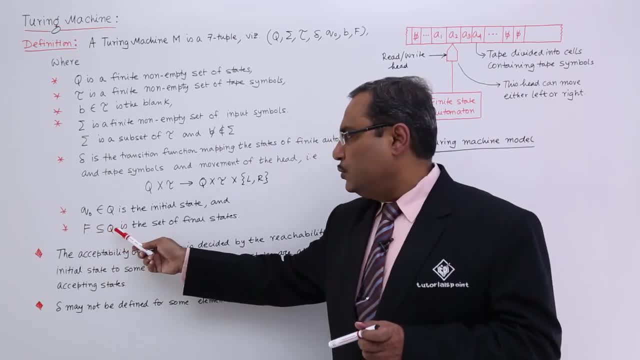 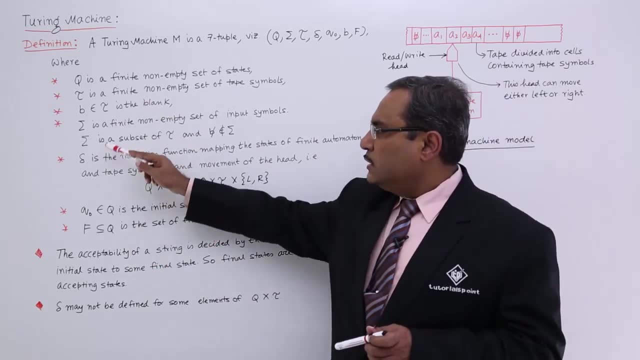 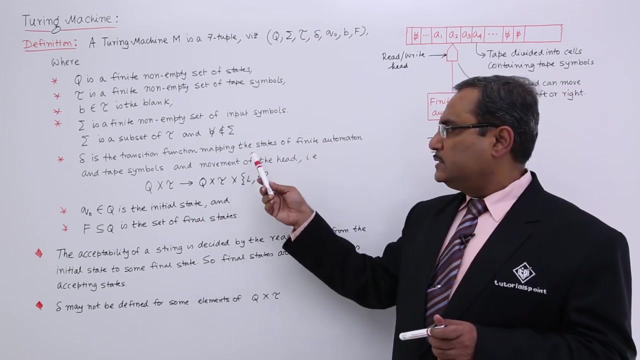 and f is a subset of, q is a set of final states, So that is a subset of q. So in this way all the 7 tuples we have defined For this particular Turing machine. obviously their conception will be more clear if you. 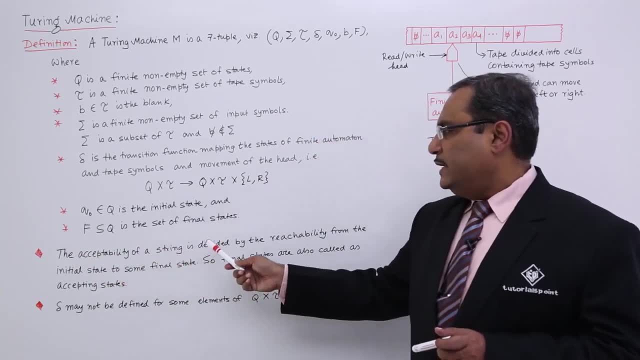 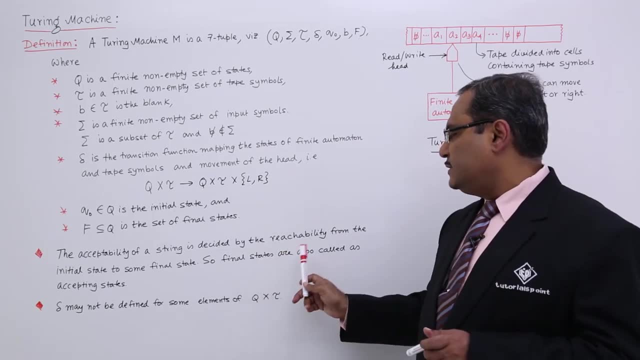 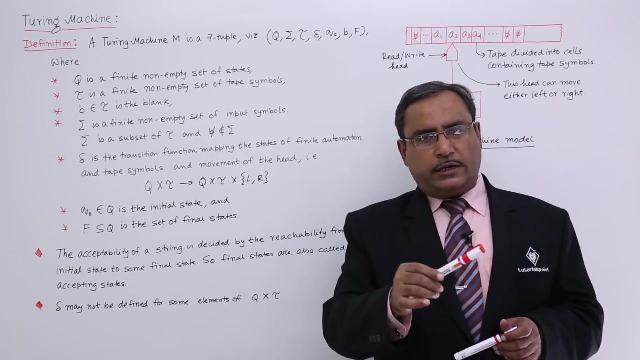 go for the example, The acceptability of a string is decided by reachability from the initial state to some final state. So final states are also called as accepting states. So reaching from the initial state to the final state for a certain input, then you shall say that the input string has got accepted by the unlock vezing, which is cruel. So this structure has got accepted by theкольarization of a string for a given state. B vagu excellence of the intelligence processes, So reachability from the initial state to the final state for a certain input. then we shall say that the input string has got accepted. 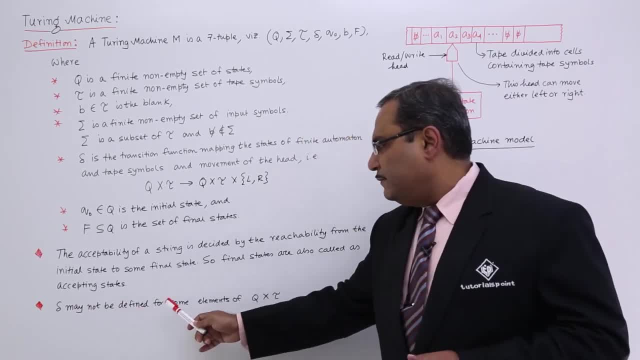 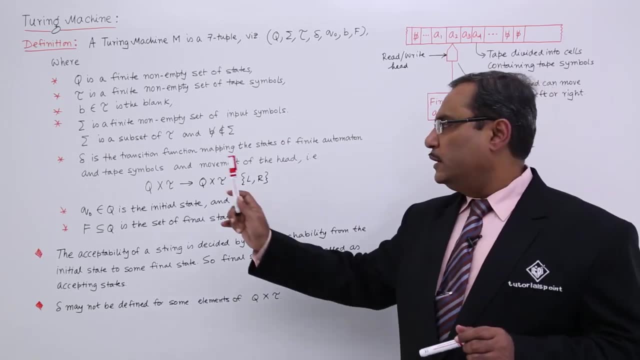 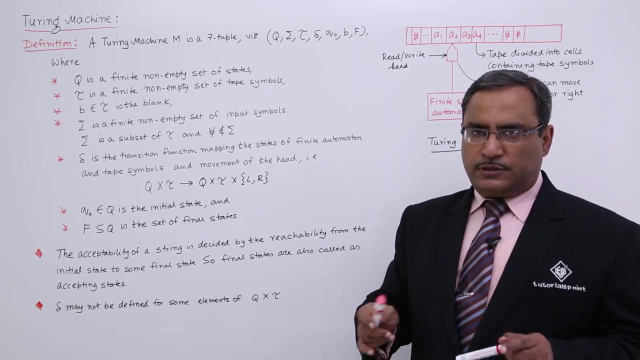 by the turing machine. delta may not be defined for some of the elements of q cross tau. so let us suppose we are having three q elements and four tau elements, so q cross tau can have twelve combinations out of them. for certain combinations the delta might not have been. 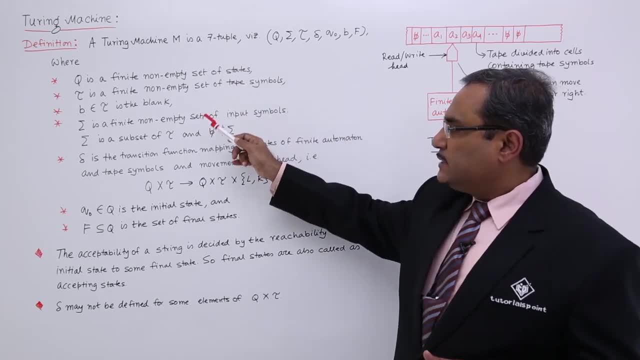 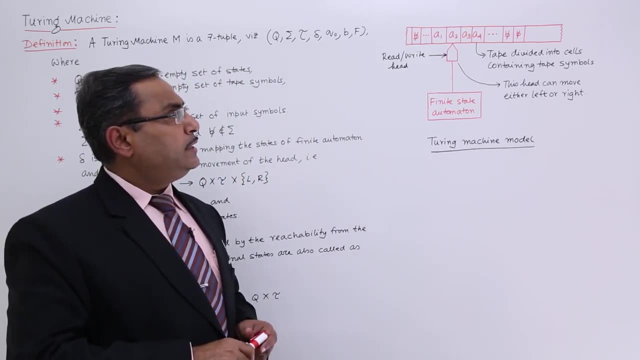 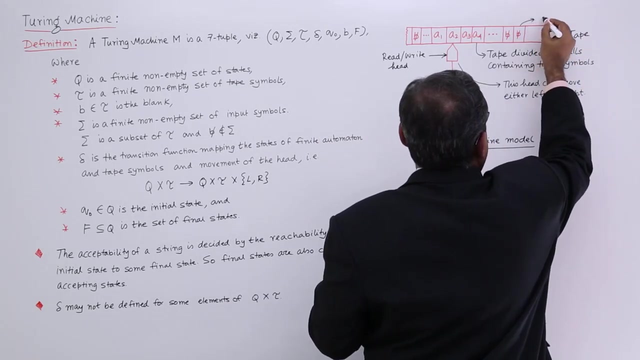 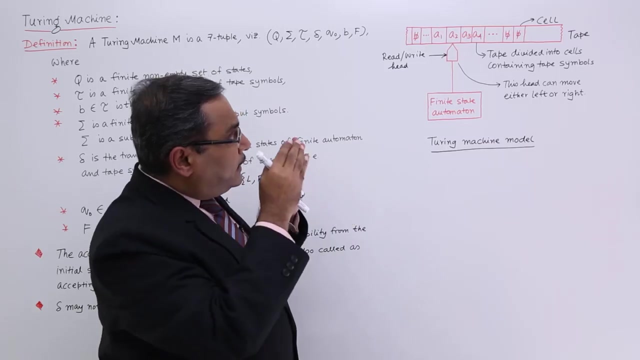 defined, so it is mentioned in that one. so this is the definition of a turing machine. so let me come with this particular diagram. so here you see, there is a tape, this is a tape and these are the cells. the tape will have some finite length and this, these are the cells, are there. each and every cell will contain. 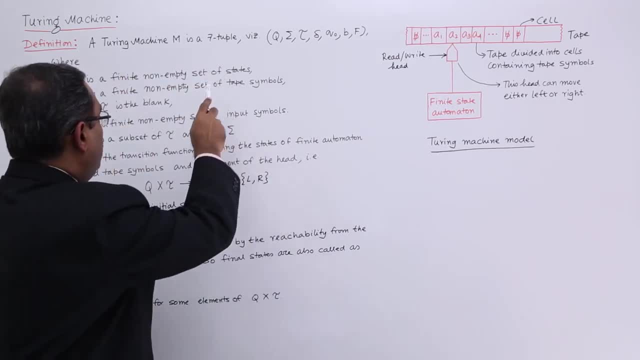 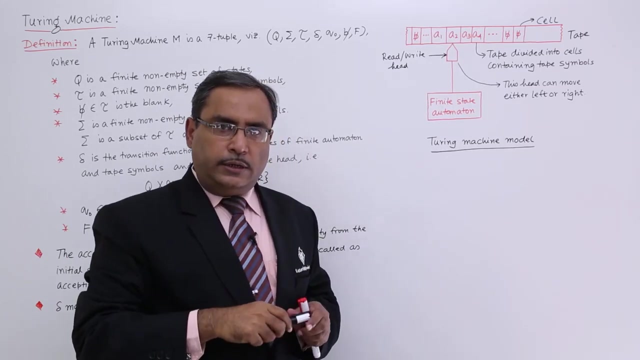 some symbol. we know that in case of tau the blank is also allowed. the blank is also allowed since in case of tau. so i am just representing blank so that i can have the parity. ok, so blank is also allowed in the, in the tau, in the tape symbol. now let us suppose there is one input. 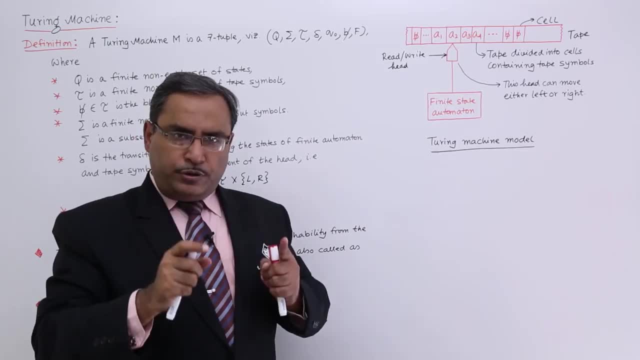 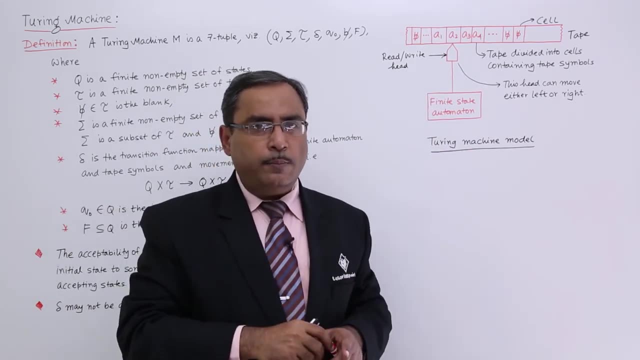 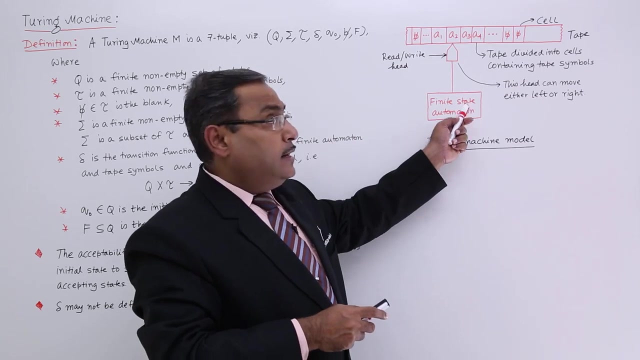 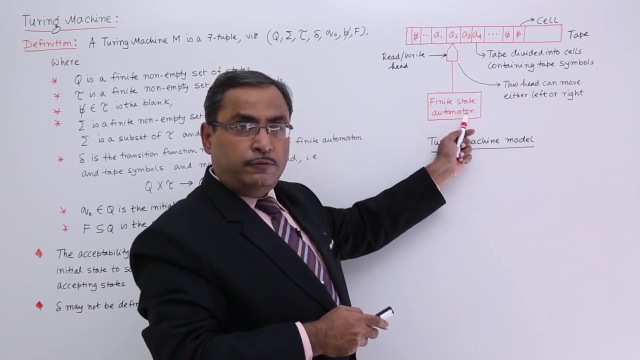 string a1, a2, a3, a4. input string can be the characters, can be also of the tape symbols, obviously, but input string cannot contain blank space. so this is my finite state: automaton. so depending upon the current state, depending upon the symbol read, i shall decide the next state of this finite automaton. finite. 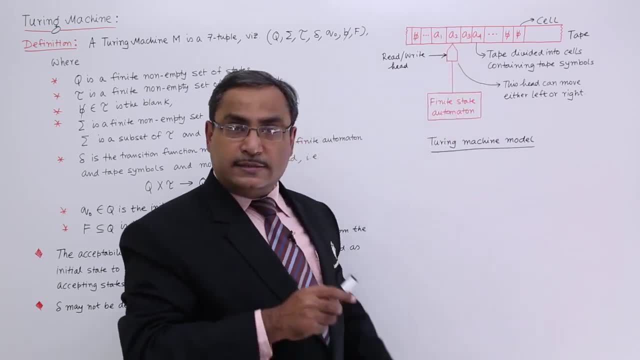 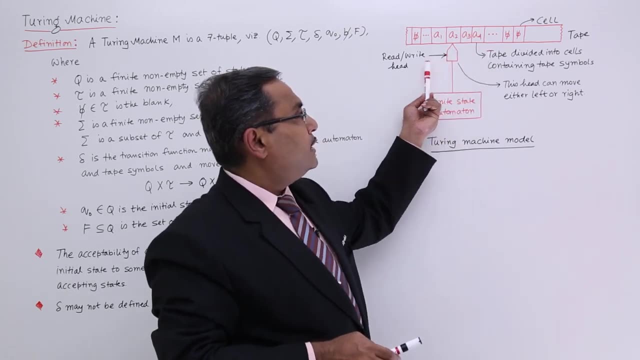 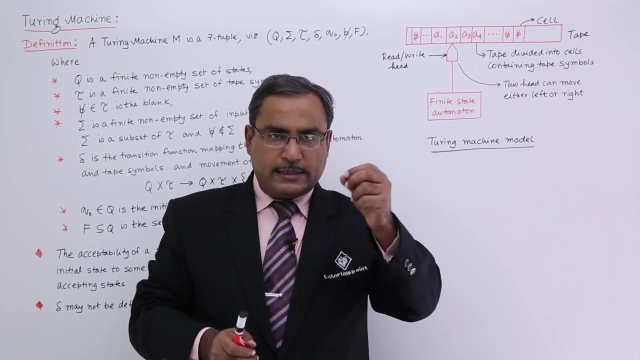 state automaton symbol to be written to this particular cell from where the symbol was read and now the reader head movement either towards the right or towards the left. that means two things will decide three things. just listen, two things will decide three things. what are the two things? the present state. 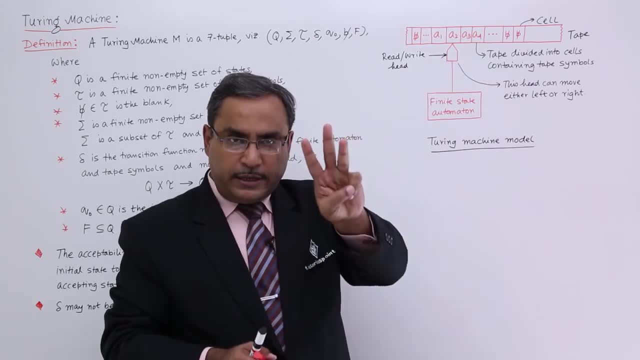 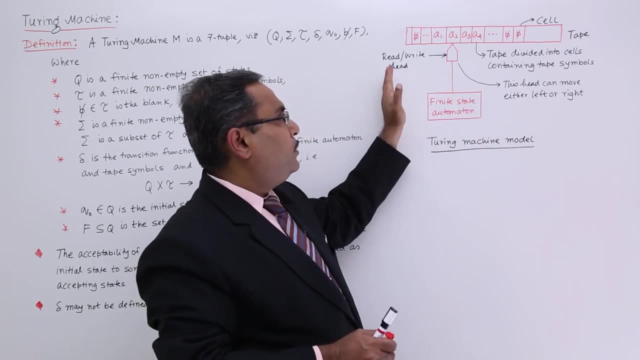 present state and the symbol read from the cell. and what are the three things? next, state, symbol to be written there and movement of the read read head either towards the left or towards the right, and that that is why the transition has been defined in this way. how many elements? 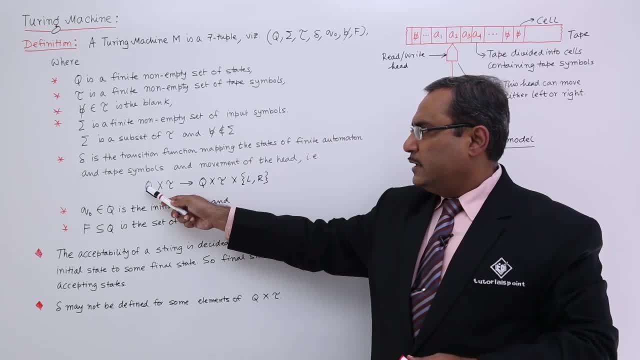 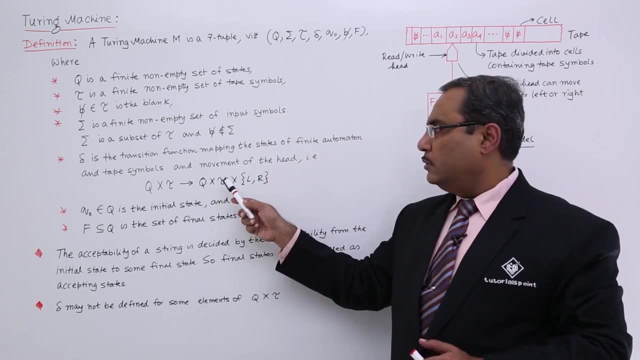 are there. we are having the two elements, one from from the state and one from this particular tau symbols. and we are having the next state, the symbol to be written on on on to the tape, and movement of the read read head either towards the left or towards the right, and 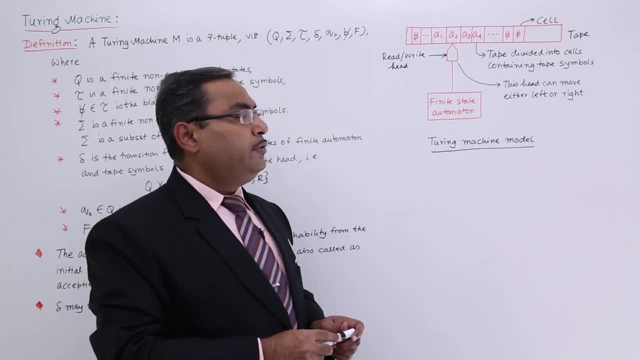 from the state, even though this state is expressed from both the individual target changes. there is no benefit of similar state. those are identical. if we are giving a state like that here, you no two part. structure was a product and once that particular state is expressed, then the manner, the atmosphere will be the one which is an impact. that 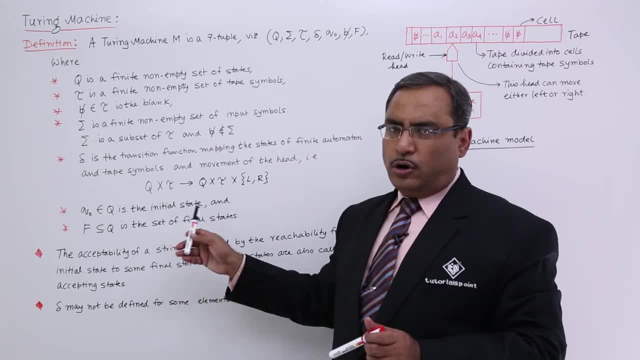 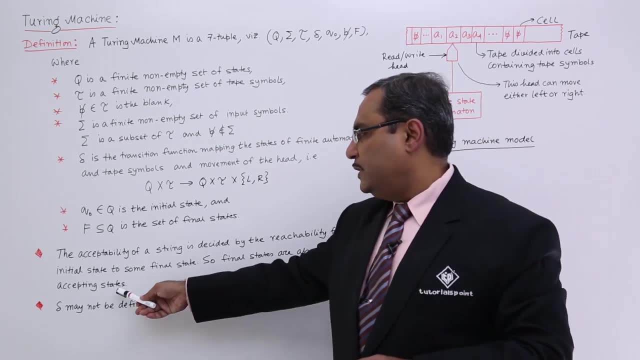 effect and we might say the state is not recreate back of the original state because we already do not use theinn 4 about 6 message, but it is there. however, if first of all state constant the state to be very другие, then that particular state will remain. 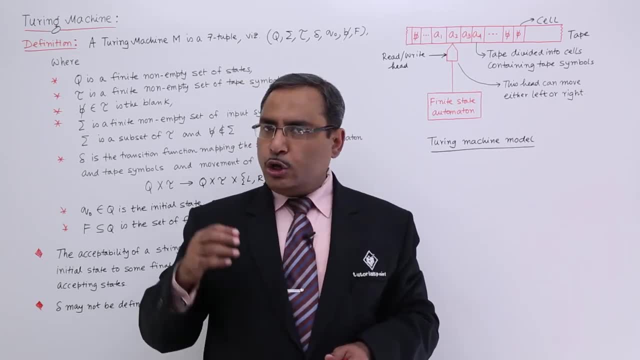 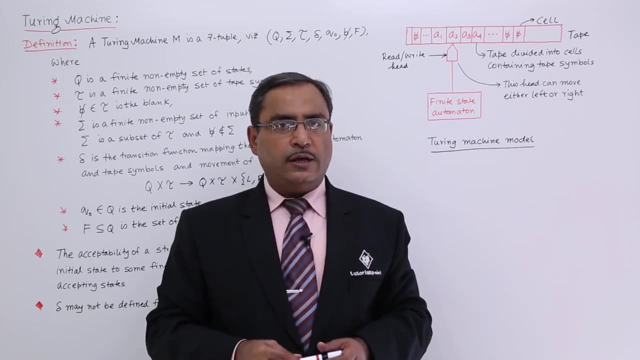 existent and we are coming to final testing and the shape of that box later as well. so the 180 26 cépte in the continuation of this one. Thanks for watching this one.